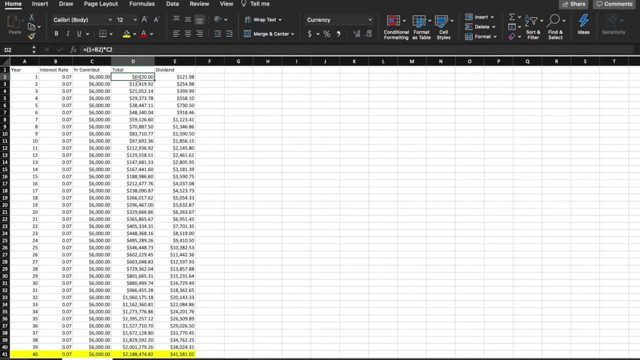 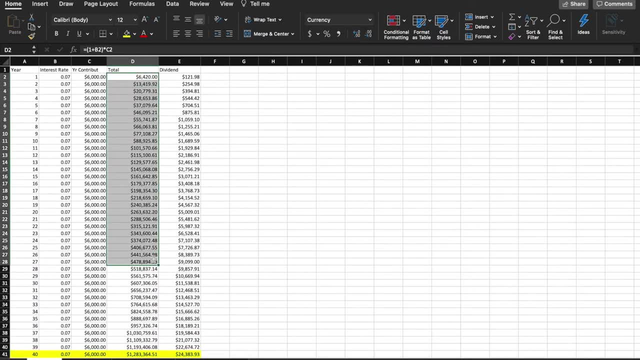 the 10% that you're putting away of your salary, of your post-tax salary. So over here, what you can see is this exact chart and you can see the total increase over time until we're saying: this is if this was retirement age, And you can see that if 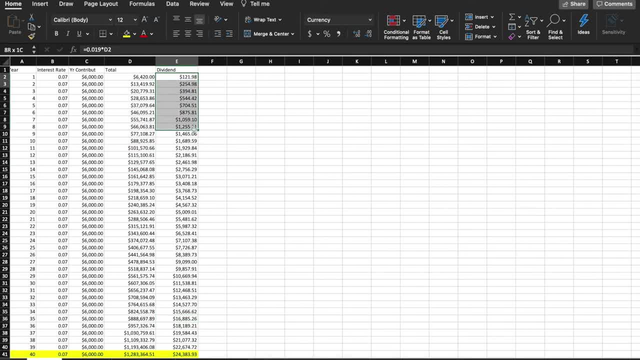 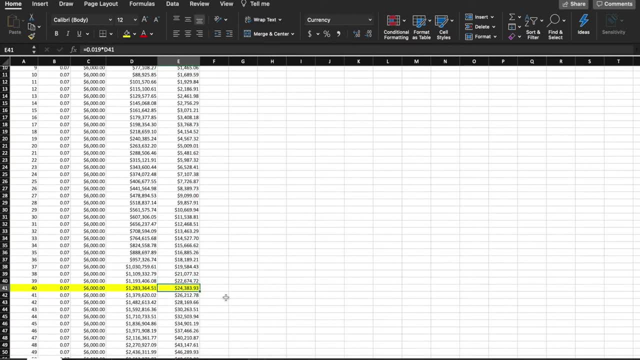 you collect, if you start contributing, you're going to start receiving checks every single year And what you're going to see is that these checks increase over time And by the time you retire, you're actually making $24,000 a year by just holding on to this money. 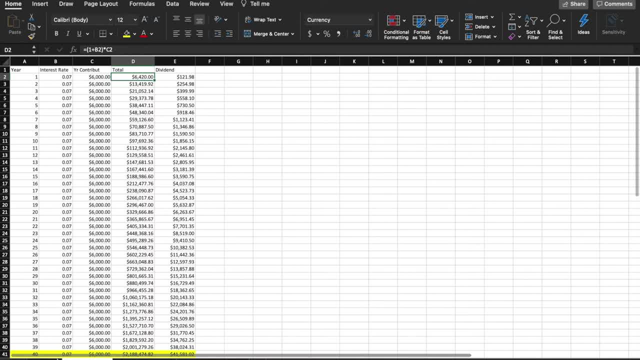 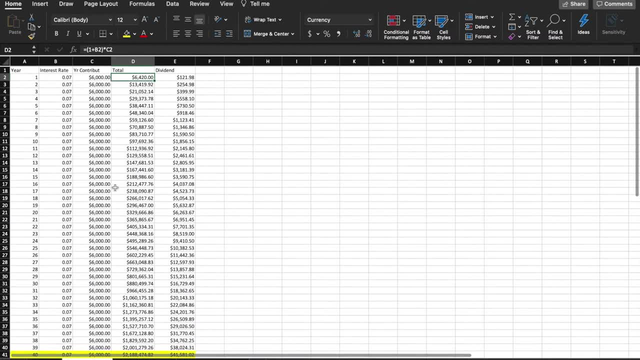 Now, if we come over here, what we see is, if you go ahead and, instead of just collecting these dividends every single month, and you actually reinvest them in something called a dividend reinvestment plan or DRIP investing, you can see that your dividends are approximately. 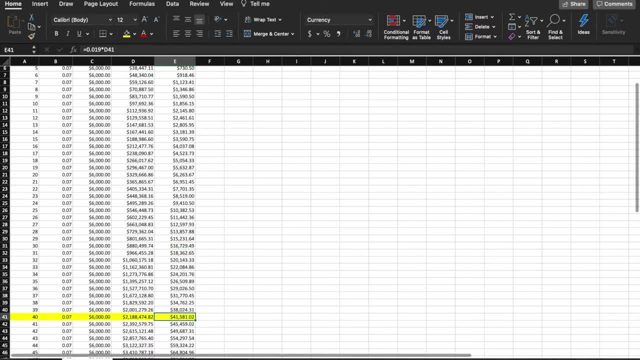 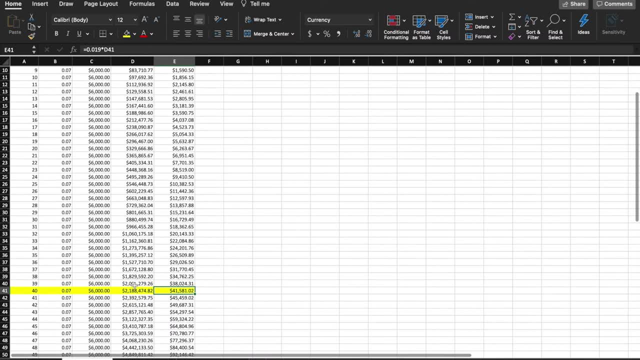 it's almost double. your dividend income is almost double what you would get as if you were to- just if you were to- just collect your dividends every year. So that's, and the other thing is that your principal is actually almost double as well. 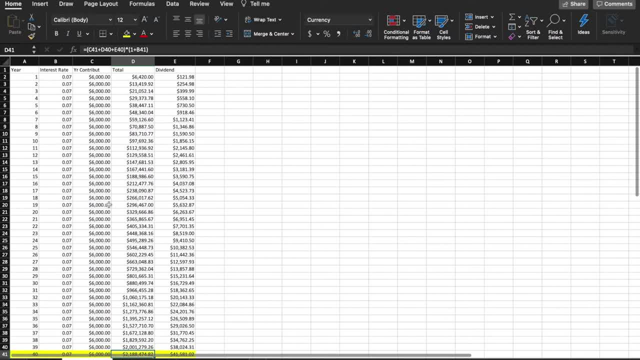 the total amount of money that you have after you're done. Now, let's say that you want to be a little bit more aggressive in your approach to investing. Now, instead of just taking 10% of your salary, let's say that you want to take 50% of your. 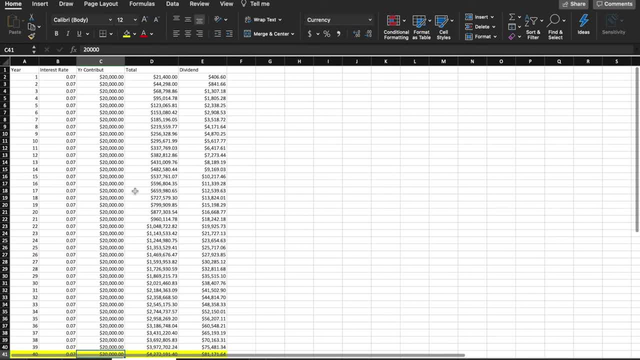 post-tax salary of the average salary That'd be around, we're assuming maybe you're paying 20% in taxes, So $50,000 salary turns into $40,000 a year And somehow, aggressively, you're going to save 50% of your dividend. 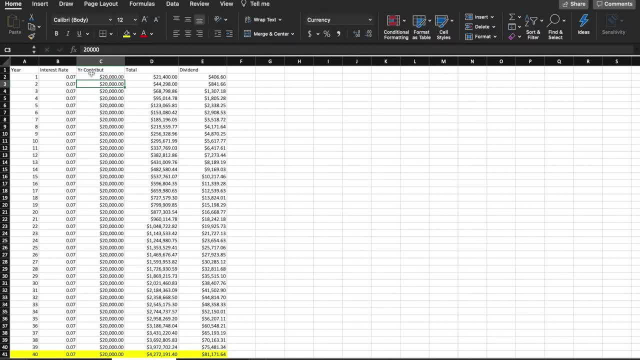 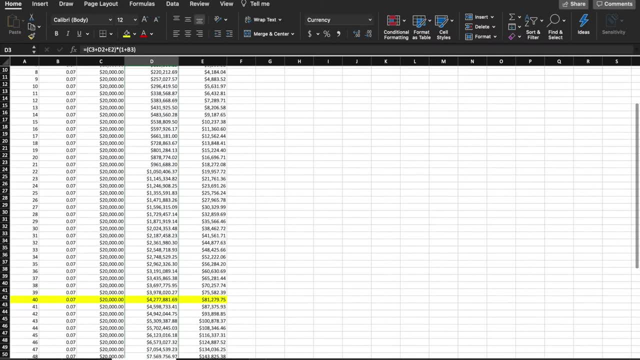 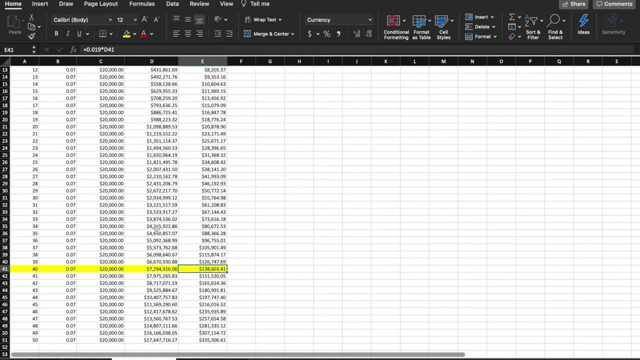 You're going to save 50% of that and you're going to invest it. So what would that look like Now, assuming that you reinvested that money? it would look a little bit different than this right. It would actually look something like this: where you're making by the time. you retire. if you reinvest these dividends instead of collecting them, by the time you retire you'll have $138,000 a year in passive dividend income, while having a principal of around $7 million. Okay, And we're assuming, right, we're assuming inflation is 3% and you're investing this. 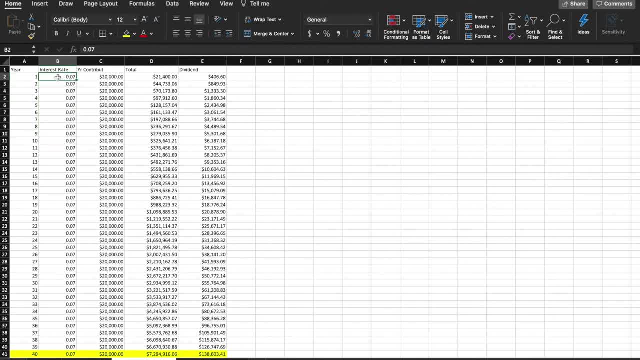 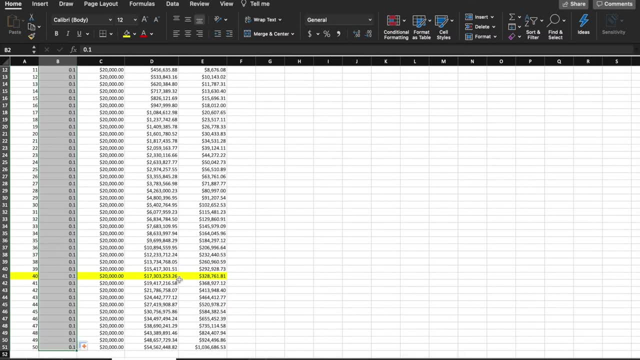 in an index fund which is getting 10% a year. So the nominal amount of money that you would have. if we calculate this real quick, we can see that the nominal amount of money that you would have by the time you retire is absolutely insane, right? So $17 million, $17 million. 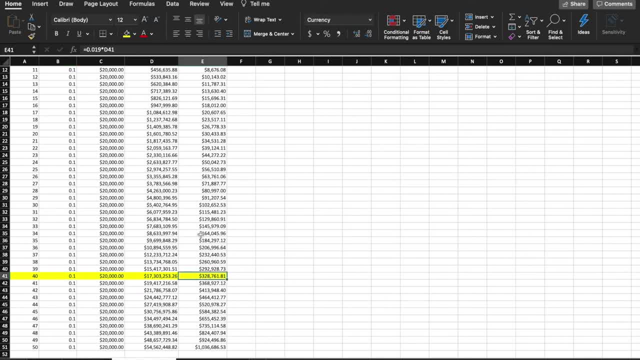 in net worth and you have a passive income of $328,000 a year. Now, of course, you know that's that number doesn't mean that much. This is the number that actually means something, because you'll have $7 million of today's buying power and $138,000 of today's buying. 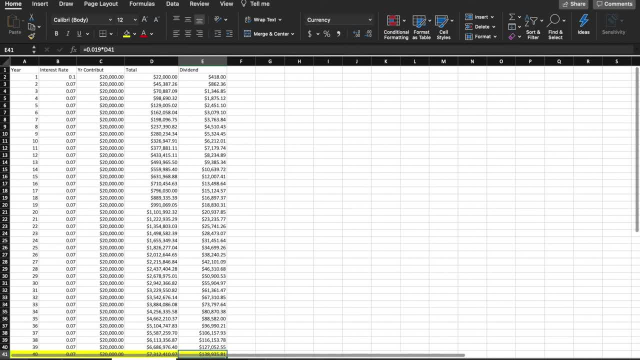 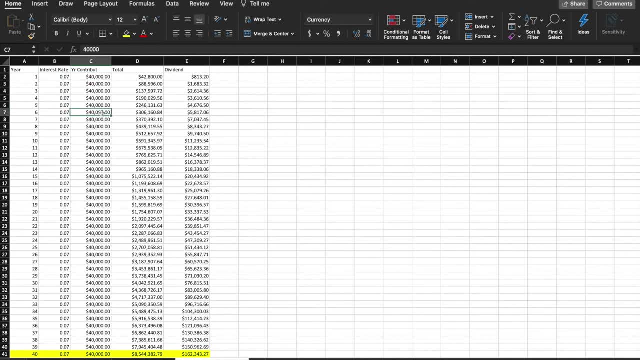 power. So that's interesting. Now let's look at another salary chart where we can look at an individual who had a high income earner, who was conscious and very disciplined with their investing. And same assumptions over here: 7% 50 years after 40 years of investing. 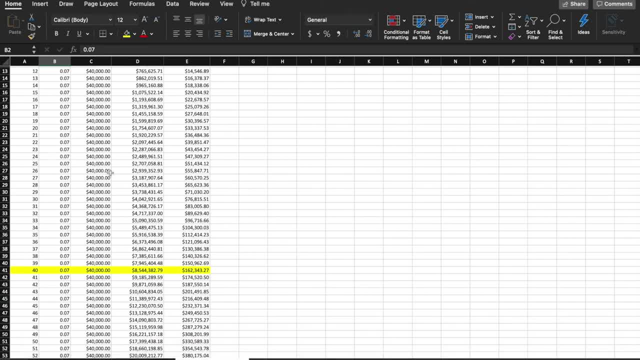 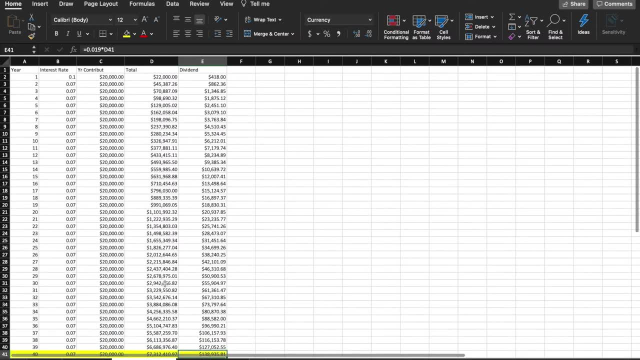 you're going to retire in your early 60s. Okay, So you know. what we see right here is without dividend reinvesting. this high income earner is actually without without drip investing. I'll show you in a second what it looks like. 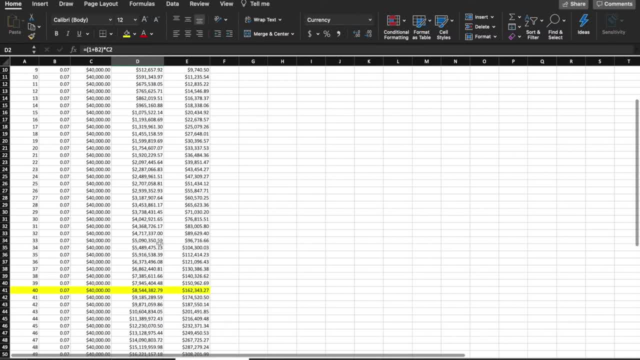 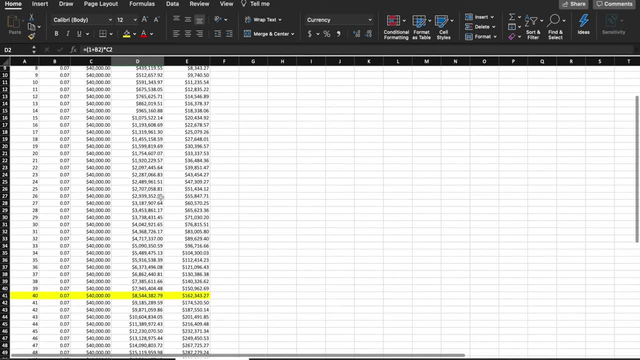 with drip investing, but it's actually making around the same amount of money as someone who did the exact same thing but didn't reinvest their dividends, which is which is crazy. So reinvesting your dividends nearly doubles the net worth And it also doubles the dividend. 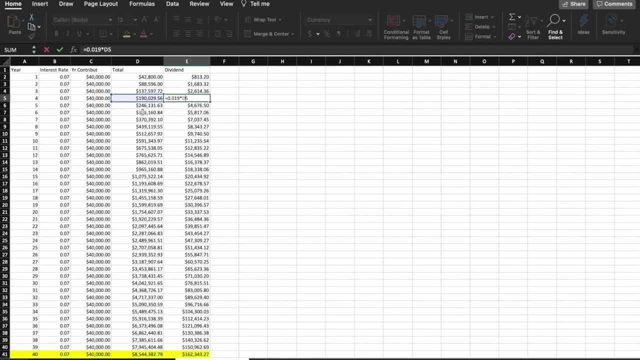 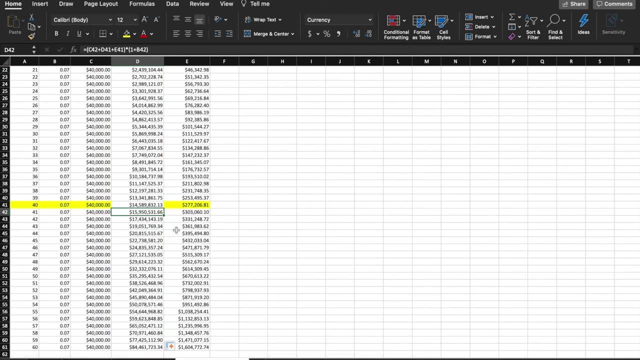 income, because the dividend income is just a percentage. It's just 99% of the total amount of money you have. Okay, So let's go ahead and we'll look at what this looks like with dividends reinvested And what we can see is that nearly 200 or $277,000 a year in passive dividend income, with a net worth of $14 million. And that is what? investing, very, very disciplined. investing, Okay, 40% of your money, I'm sorry, 50% of your post-tax income, year after year after year. 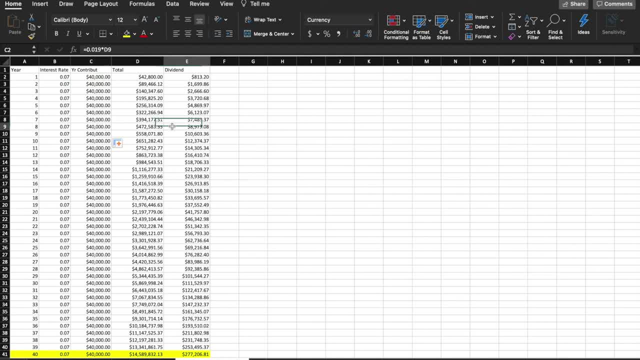 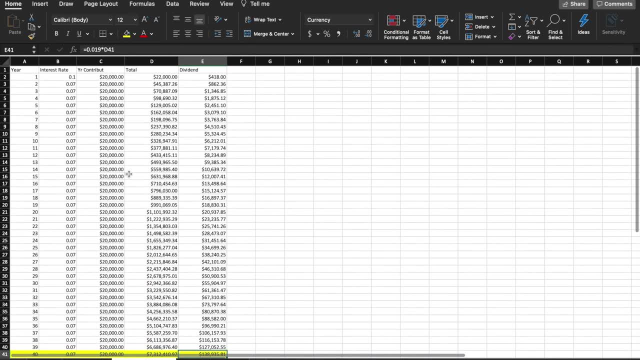 until you retire is going to be. maybe all this does is maybe it is incredibly impractical to save 50% of your post-tax income year after year after year. Um, you know, especially if you're living on $50,000 a year with a family, if anything. looking at these different, 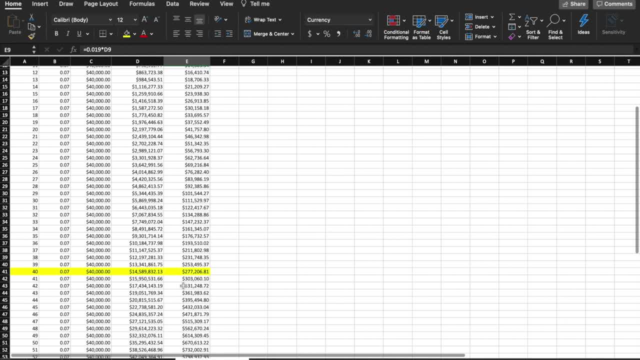 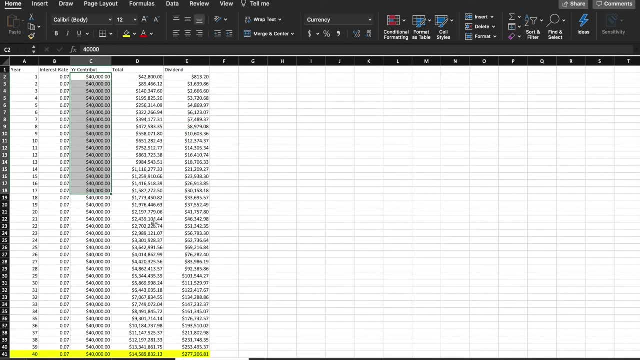 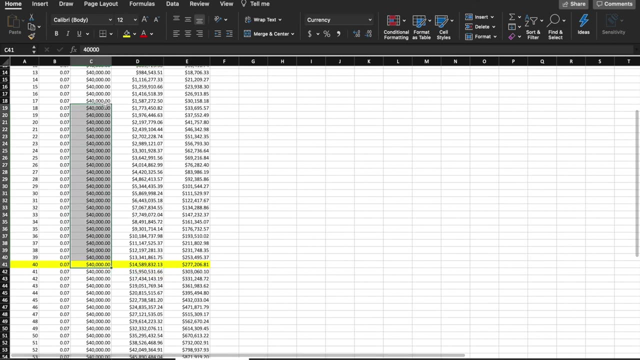 scenarios and savings rates has just absolutely inspired me to save and to see just how much saving money early on really really matters. And you know, you can even like if we just delete all of these contributions from then on, you can see your principal doesn't change. 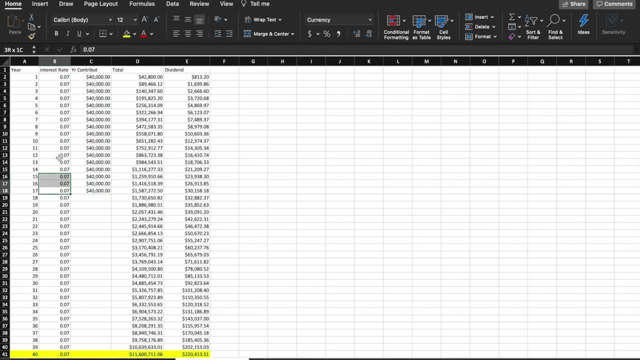 that much. It's really these early years that matter a lot, And it's also the interest rate that matters a lot. So, if anything, this just goes to illustrate the importance of drip investing, and not only investing and being conservative and um, investing as much of. 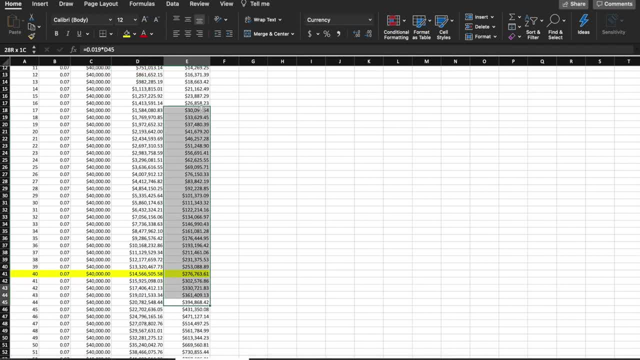 your money as you reasonably can, but also the idea that you know dividends have a profound effect on your income. So it's really, really, really important- And I think that's really important- to reflect on the amount of money that you have, And it's so important. 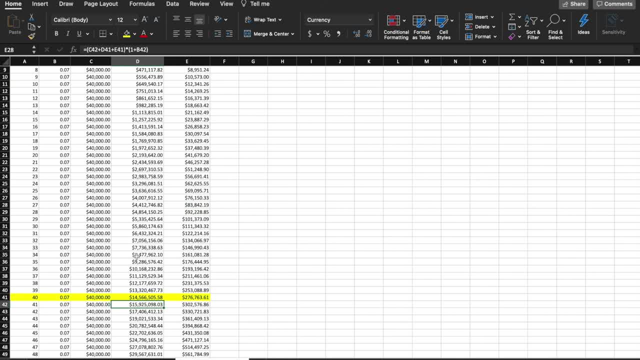 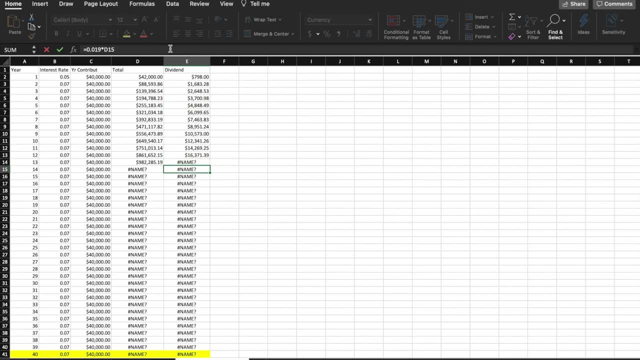 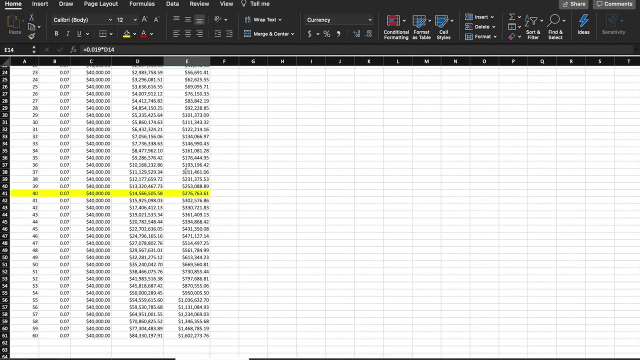 to just put those dividends and reinvest them. Almost half of the compounding that's done is done from just this 1.9% in dividends that's being reinvested every single year. So I hope this video was helpful in explaining maybe the investment process and what it looks like. 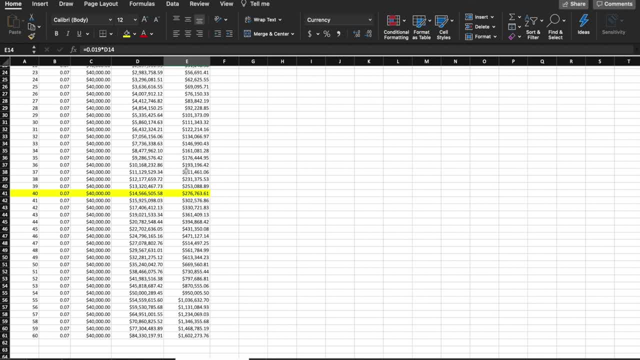 from a more mathematical perspective. Thank you for watching.